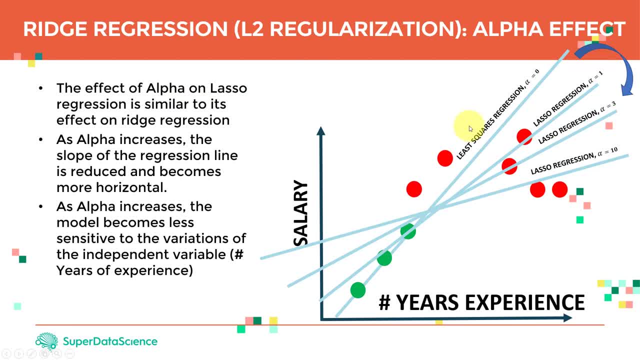 going to have the same parameter, which is alpha parameter, and as this is very similar to ridge regression, as you increase the alpha term, as the line becomes more horizontal and as you basically reduce the sensitivity of the changes in the independent variable, Okay, again, as alpha increases, the model becomes less. 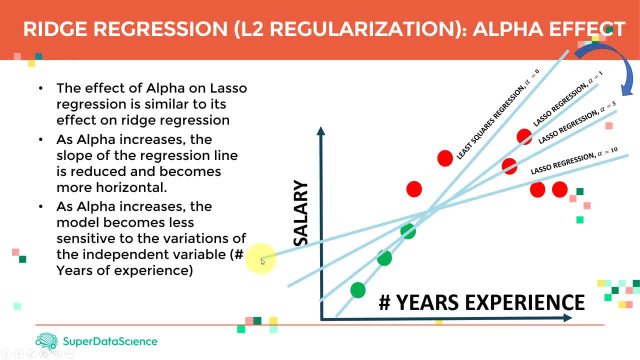 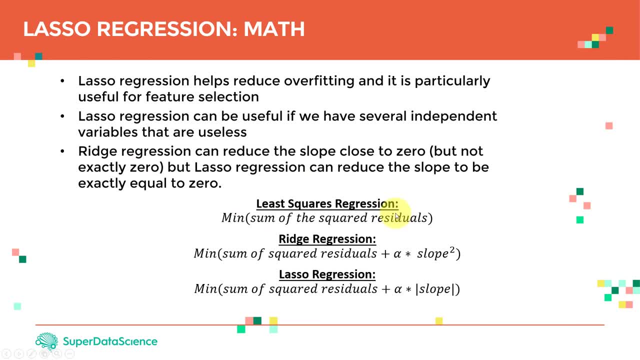 sensitive to the variations of the independent variable, which is the number of years of experience. All right, so let's summarize. so, as you guys can see here, this is my least square regression: minimum sum of square residuals. ridge regression is minimum sum of square residual. plus alpha times, slope square and lasso regression, we're going to be minimum sum of square residuals. 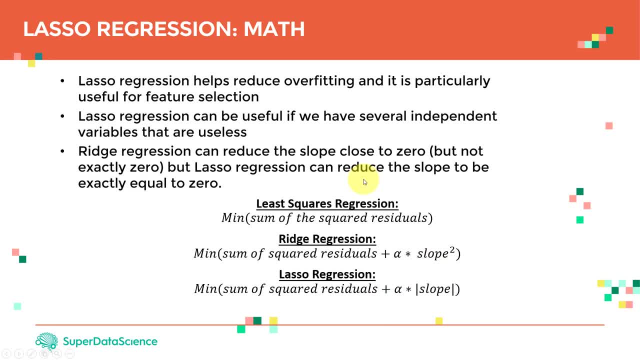 plus alpha times, the absolute of the slope. and, as I mentioned, lasso regression helps reduce overfitting and is particularly useful, mainly for feature selection. So one of the main kind of unique elements about lasso regression, as compared to ridge regression, is that lasso regression can be used for feature. 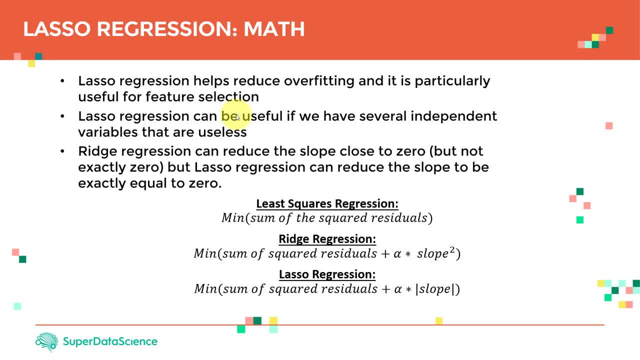 selection, which means it can give me an insight of which independent variable is actually useless. Okay, however, ridge regression cannot directly tell me this. why? because ridge regression can reduce the slope close to zero, but it's not exactly zero. it actually can reduce it, yes, but not exactly. however, why? because there is a squaring term. 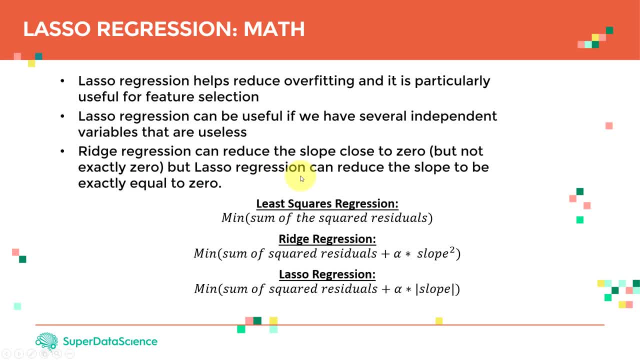 that's all what it is, however, but for lasso regression it can reduce the slope to be exactly equal to zero, and which means that I can directly eliminate some of the independent variables that are useless, and that's kind of one key advantages of using lasso regression over ridge regression. 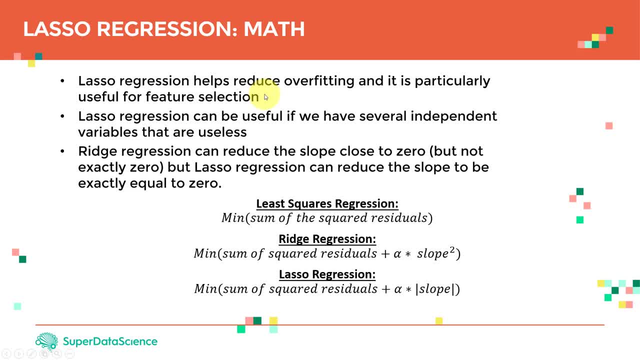 ridge regression. It can be used for feature selection and I can mainly use it to get rid of any parameters that are useless. I will only keep the parameters that are useful to me, And that's all what I have for this lecture. I hope you guys enjoyed it. 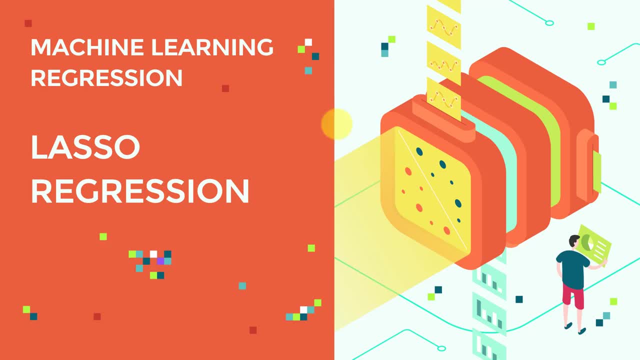 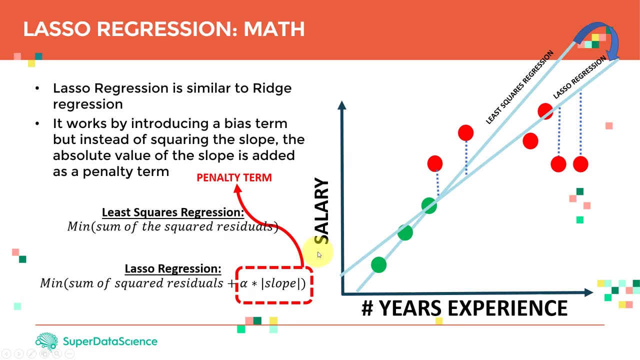 Let's recap: In this lecture we have been able to cover the lasso regression, which is again regularization technique. It's pretty much work, the same as ridge regression. We're just going to add an additional penalizing term, which is alpha times the slope of the line, absolute of the slope.